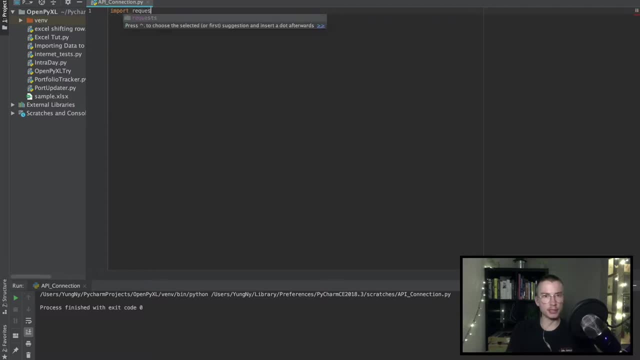 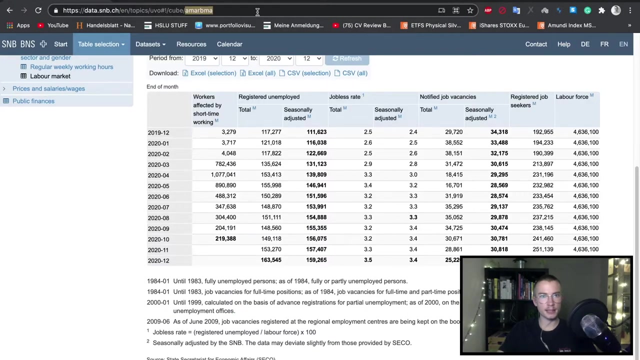 module and we would like to import requests. We would like to retrieve the data, and the data is retrieved by requestsget, and then we would like to retrieve the data as text. So, as I've shown you, we are going to copy the address into here and we are exchanging the API key with the. 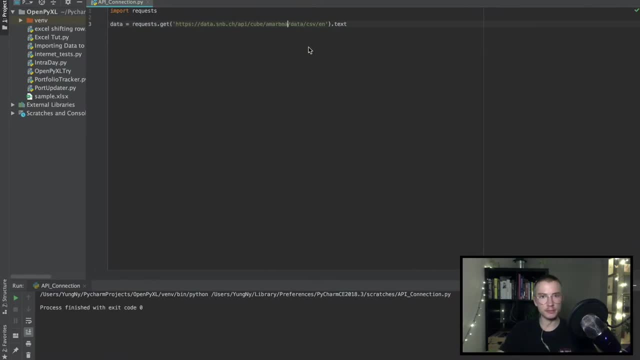 actual part that we would like to retrieve And just to check if everything works. we would like to print the response. As you can see, we got the whole table now. however, it is not formatted in the way that we would like to have it. in the end, We only want to. 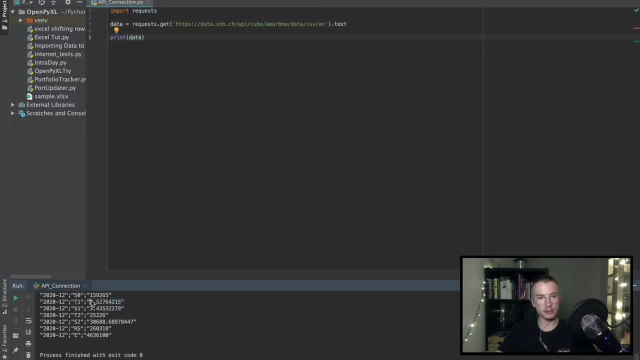 have this part, so this number actually, and thus we need to do a bit of formatting here. So let's say, the next variable is datatext and we would like to retrieve the string of data, but in this case we would like to split the lines because 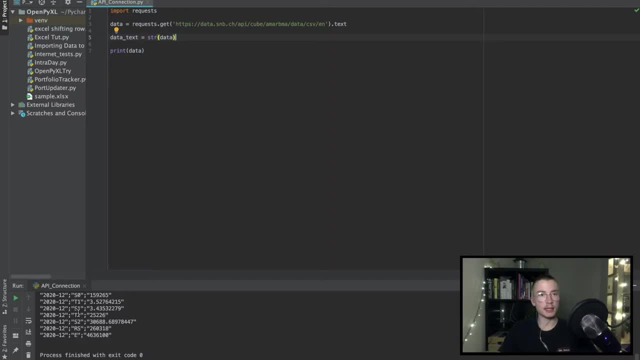 everything is separated by lines. we would like to retrieve the information just in one line and then from the list we would like to pick the specific line or the specific part of the list that is filled with our information. so this is the one, two, three, four, five, sixth line. so what we are going to do is we are 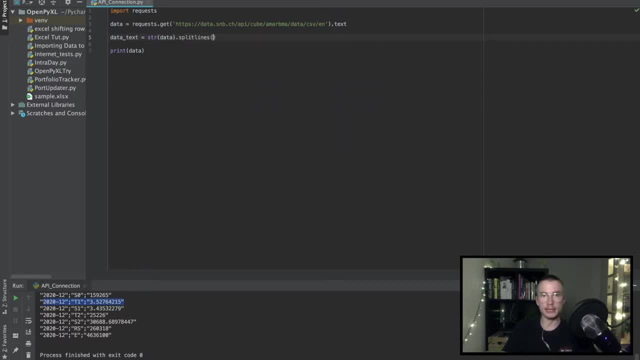 going to split, split lines, just self, and then we want to retrieve the sixth part of the list. let's see if this works. whoops. of course I would then also have to print this variable. so, as you can see, we have now just the part that inherits our information, but 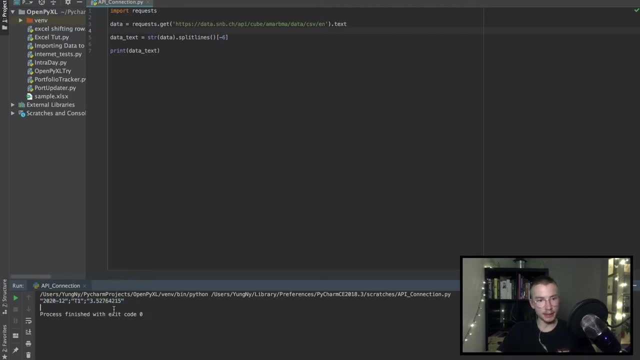 it is not quite a list yet. it is just a line and it is still delimited by semicolons. so what we are going to do is we are going to nope, we are going to split the information and we are going to split it by semicolons. so 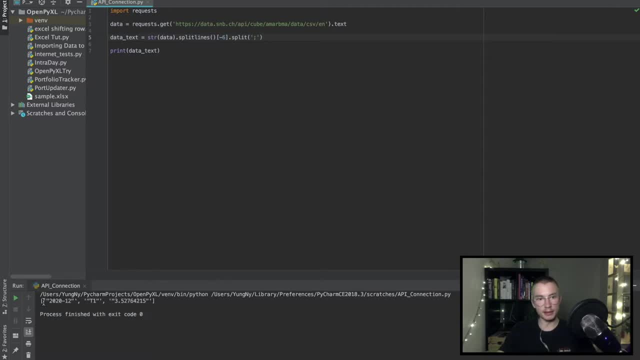 We have now a list that has three parts and we would like to retrieve the third part. As you know, Python is counting from zero and therefore, to get the rate, we want to get the third part of the list, so two. Let's print the rate and see if it works. 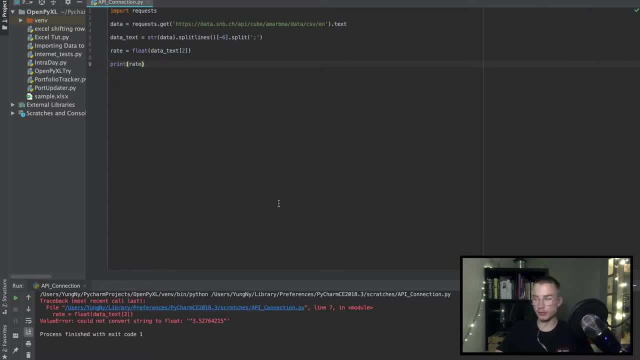 Right now we see that the part of the list still has the quotation marks in it and therefore we have to delete the quotation marks in order to make this text part a float. We do that by calling replace, And we would like to replace the quotation mark with just nothing. 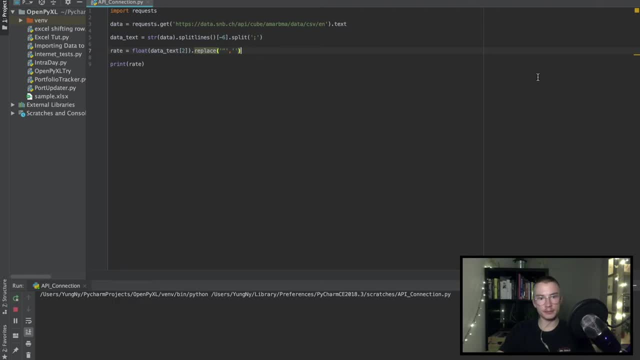 Let's see if this works. Whoops Replace. I did a mistake here. Ah, I forgot. Is that correct? Of course, we need to then delete that parenthesis And, as you can see, now we just have the unemployment rate from December 2020, as this is the latest information that we can get from the Swiss National Bank. 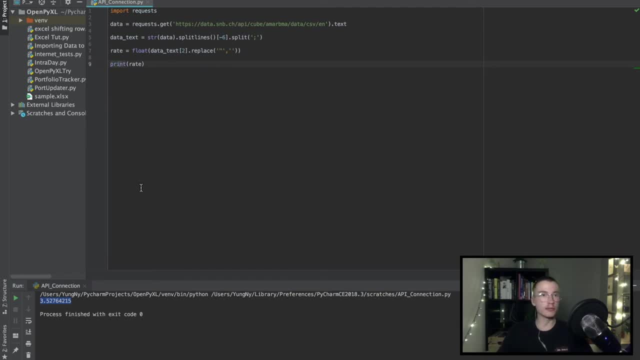 You can obviously use this to retrieve any information from APIs that you want. You have kind of seen the workflow that you need to do in order to get around some of the hurdles that you might incur, So, for example, that the data is not formatted rightly. 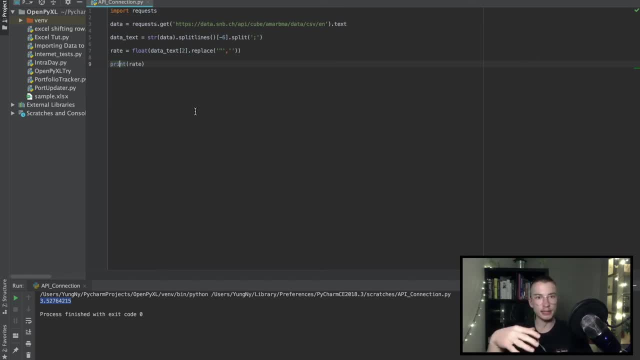 Or that the data is not at the end of the list but rather somewhere in the middle, But as long as the formattation in itself is always the same. So if the unemployment rate is always at the sixth row from the back, this will work basically forever. 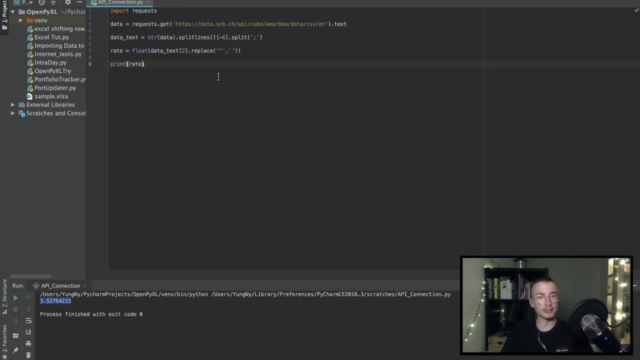 So if this has helped you, please consider liking or subscribing And, in any case, have a great week. Bye, bye, Thank you.